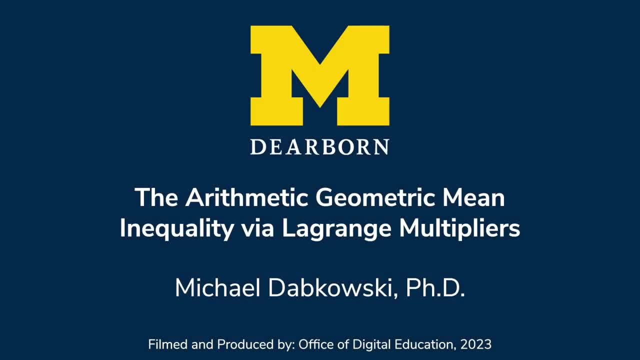 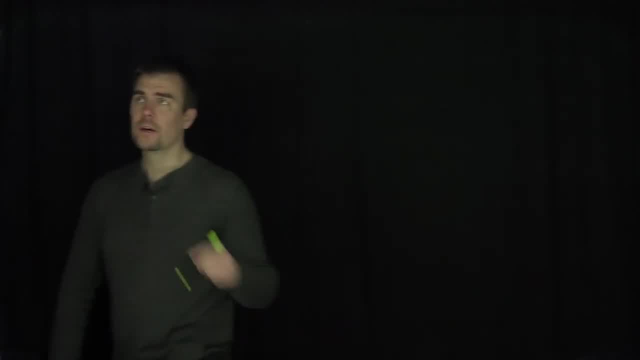 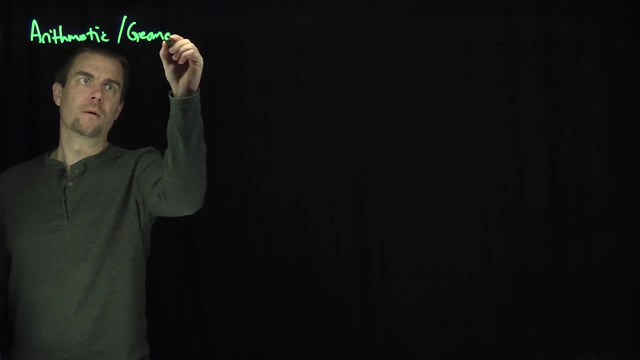 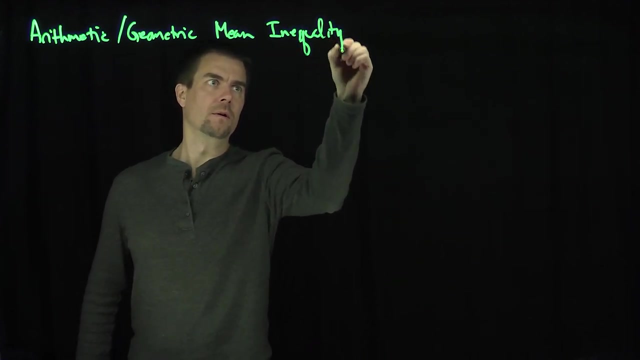 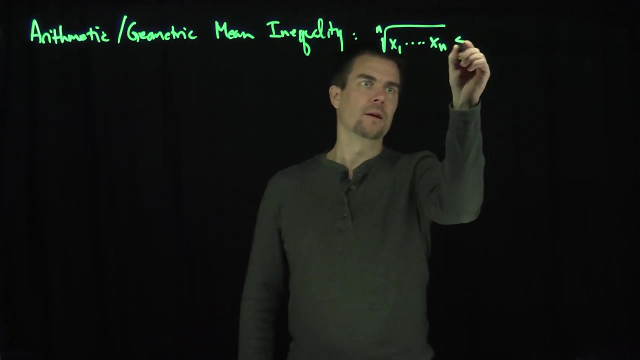 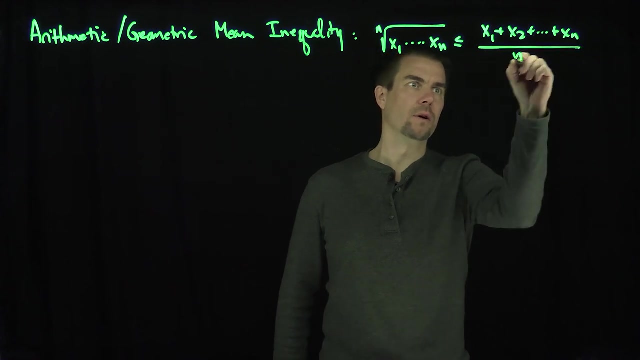 Hello students, in this video we'll prove the arithmetic geometric mean inequality using Lagrange multipliers. The arithmetic geometric mean inequality states that if I look at the geometric mean, the nth root of x1 times xn, that is always less than or equal to the arithmetic mean x1 plus x2 plus xn over n. 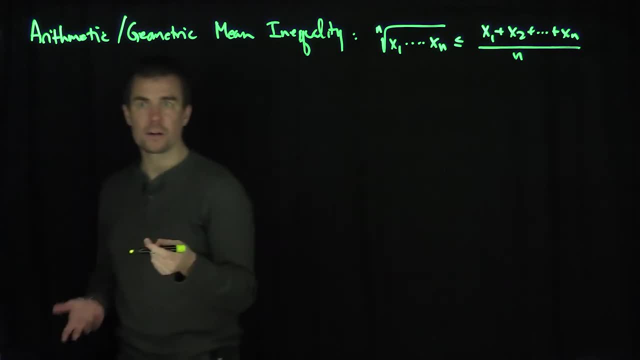 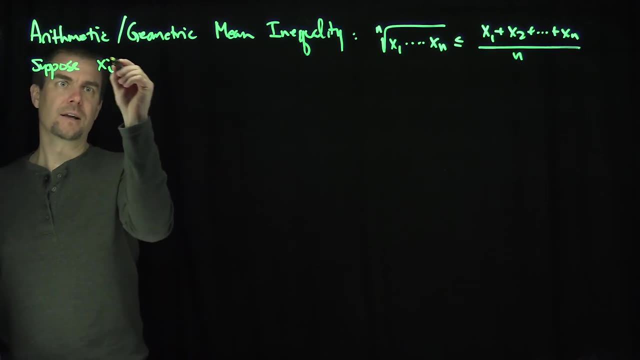 Okay, we're going to assume that the x1 through xn are not negative. in particular, we'll just assume they're positive for simplicity. So assume, suppose, that xi is greater than zero for all i, just for simplicity of my calculation. 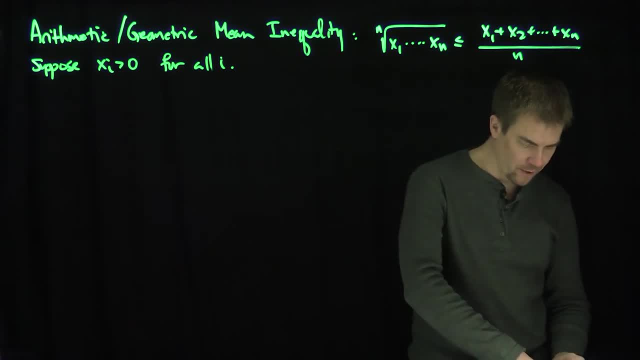 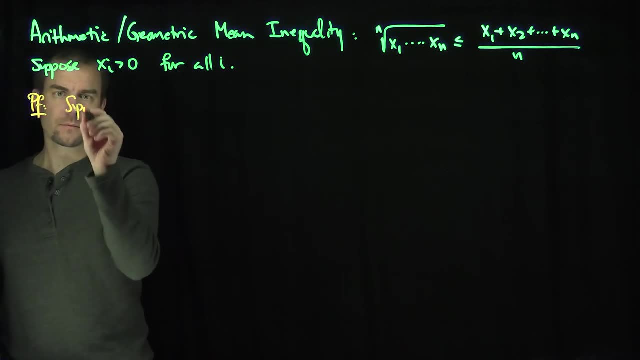 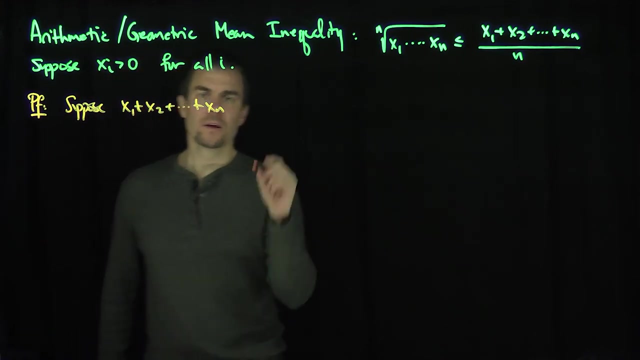 And I'm going to prove this. And so I'm going to prove this using Lagrange multipliers. and so the methodology is the following: What I'm going to do is I'm going to suppose, so here's the proof: We're going to suppose that x1 plus x2 plus plus xn is equal to a constant number. I'll call it a right. 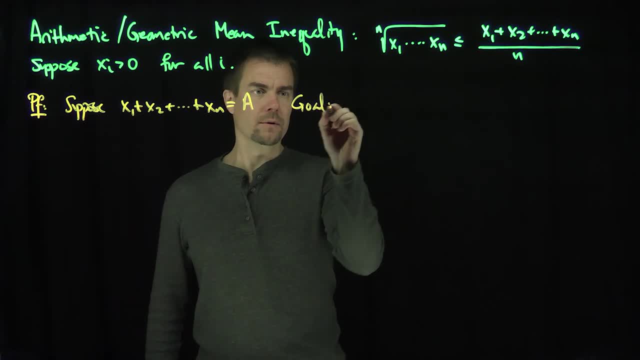 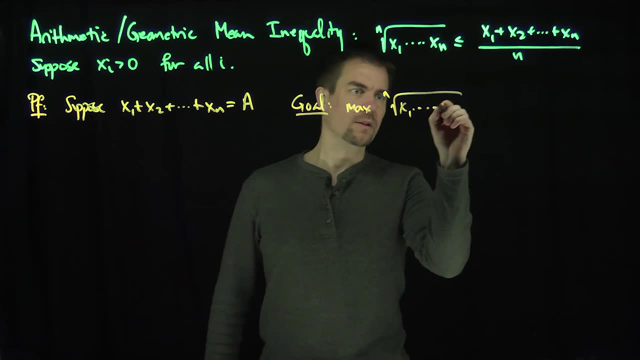 And I want to find the maximum. my goal now, my goal is to find, is to maximize, is to maximize this function, which is just the nth root, nth root of x1.. x1 times all the way down to xn. 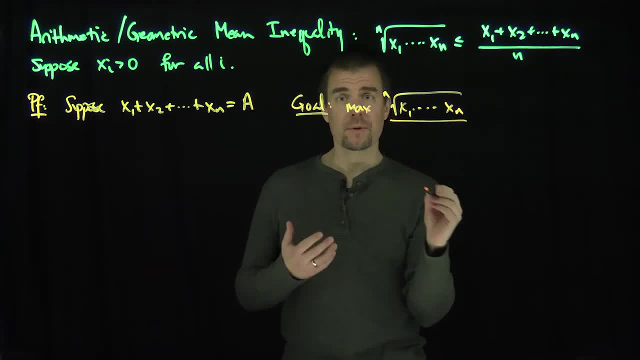 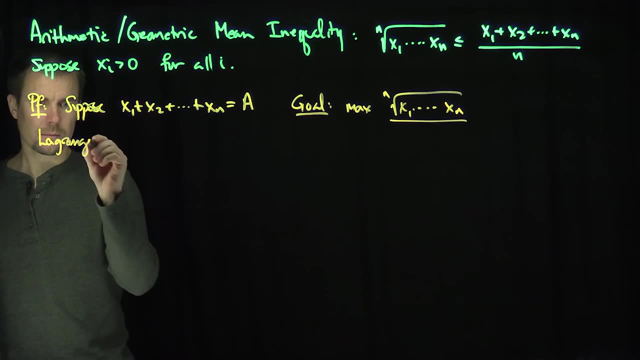 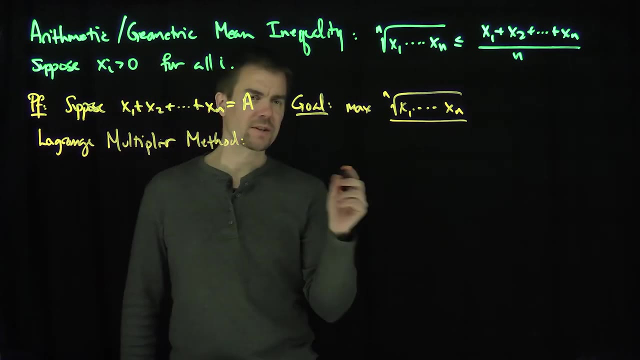 All right, and so now we're going to use Lagrange multipliers. I'm trying to find the maximum of this function. I'm going to try to optimize this function subject to this constraint. So the Lagrange multiplier problem states that the gradient- so let's call this function over here- f of x1 through xn. 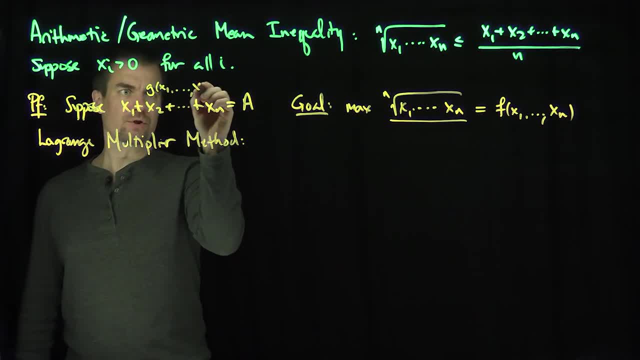 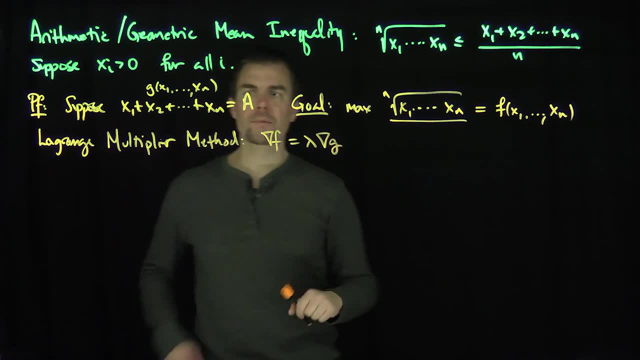 and let's call this constraint over here this sum, and in g of x1 through g of xn. So the Lagrange multiplier method says that the gradients of f is proportional lambda to the gradients of g right, And so of course the gradient g is elementary to compute. 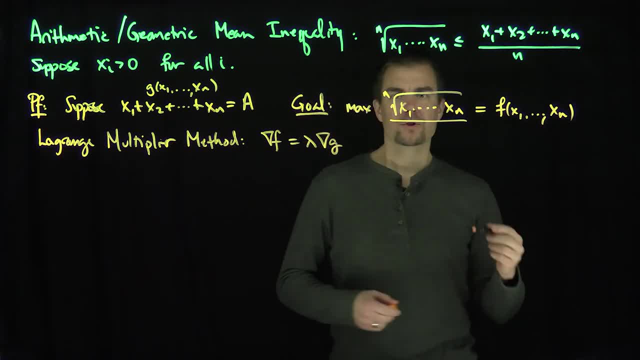 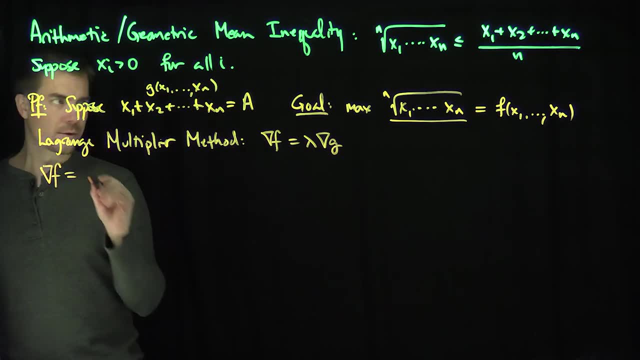 The gradient of f is only slightly more difficult to compute. so what is the gradient of f? So note in particular that it's a symmetric expression. so what I can say is I can say that the gradient of f, the gradient of f is going to be well if I do the derivative with respect to x1,. 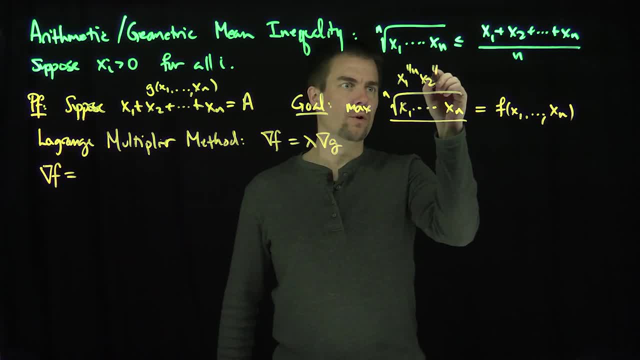 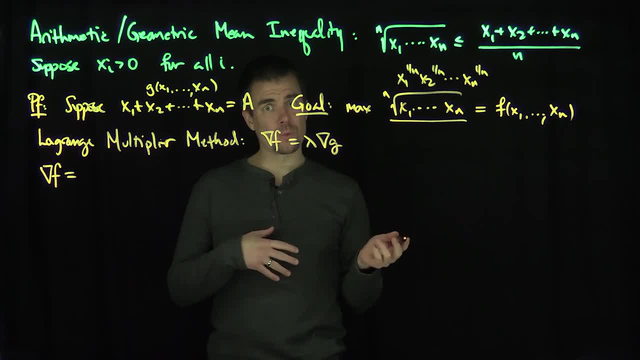 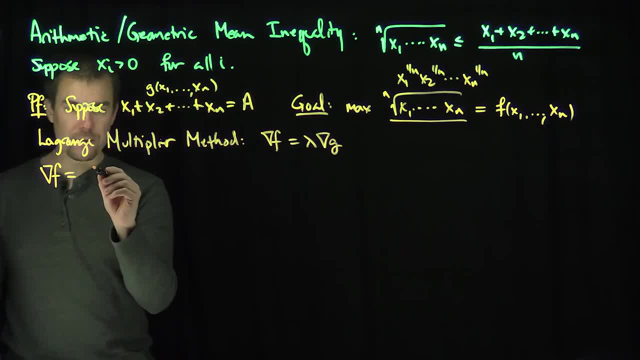 And so I see that when I do this, I'm going to get a copy of f itself, and then I'm going to have a 1 over n in each term, 1 over n, x1 to the negative 1,, 1 over n, xn to the negative 1, okay, 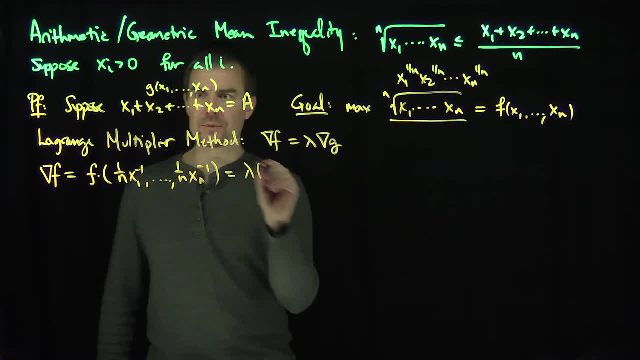 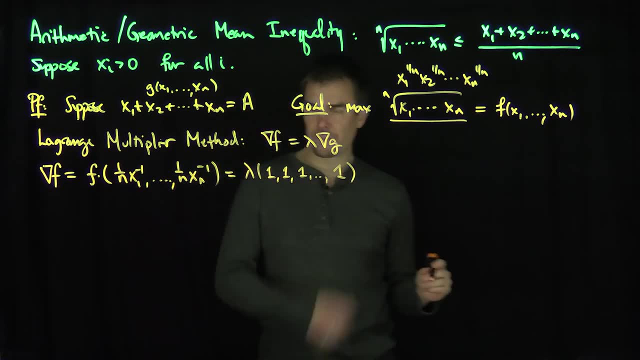 So that's a scalar and that's equal to lambda times the gradient of g. that's even easier. just all 1s, 1,, 1, 1,, all the way down to 1.. And so my conclusion from this is that what 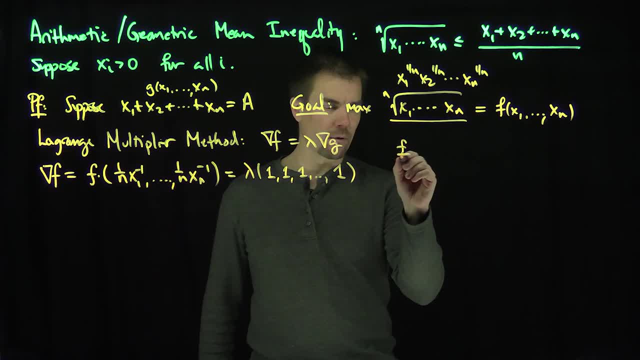 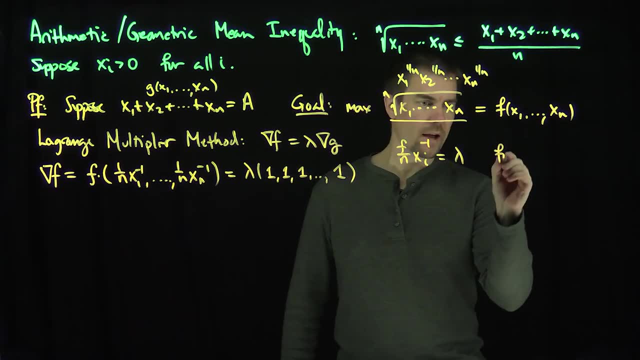 My conclusion is that, if I look at f over n, f over n, xi is going to be equal to lambda for all i, to the negative 1 for all i. So, in particular, what this says: since f is not equal to 0,. since n is not equal to 0,. 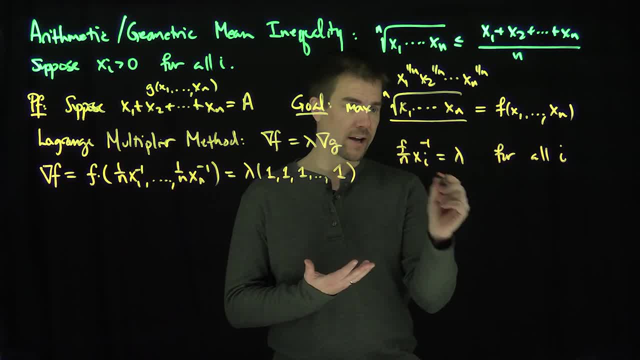 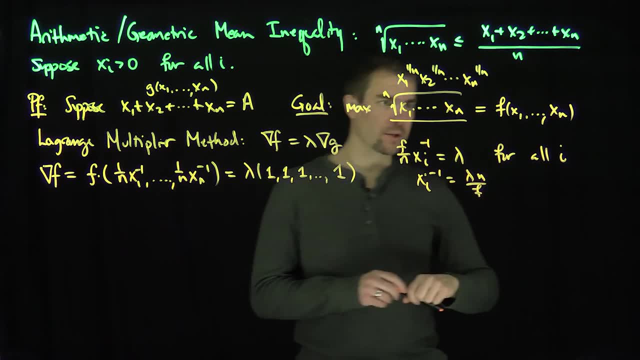 this condition over here says that xi has to be equal to xj, since all of these xi inverses. so in other words, this would say: xi inverse is equal to lambda n over f, since f is not equal to 0,. 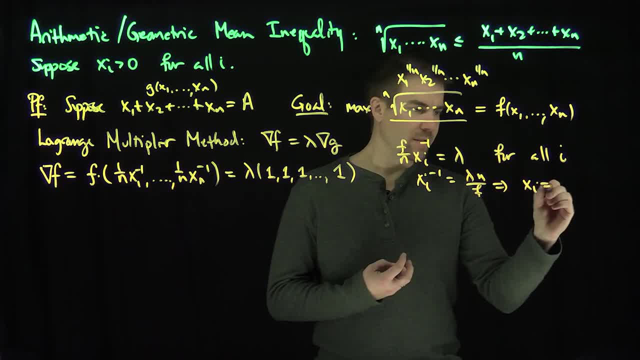 and then that forces all of these xi to be equal. so xi is equal to xj. That's what we get for all i and j, so all of them are equal to each other. And so now what we can do is we can look at the constraint equation. 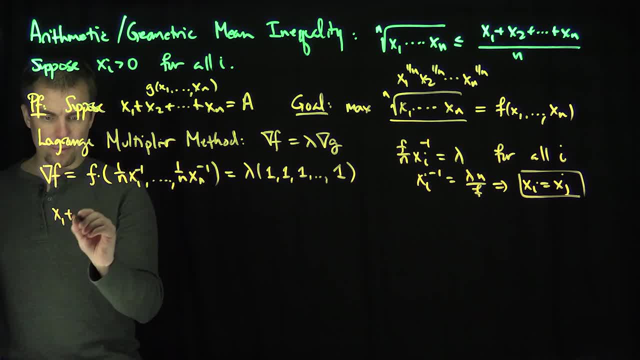 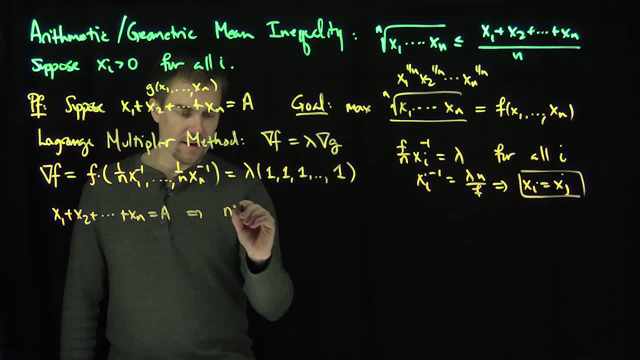 So if all of the xi are equal to each other, then the constraint equation is: x1 plus x2 plus all the way down to xn is equal to a. all of them are equal. so the constraint will imply that n times x1 is equal to a. 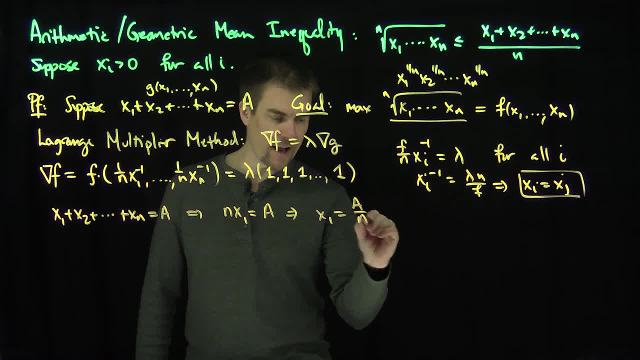 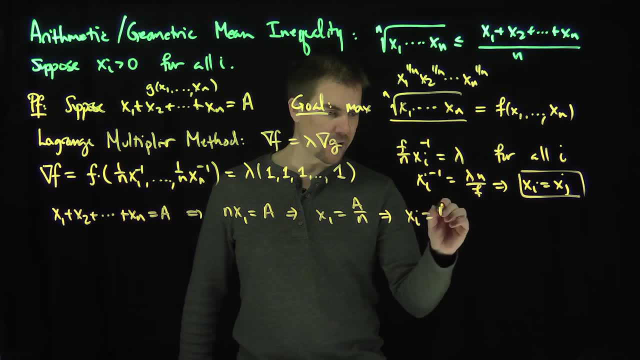 so that says that x1 is equal to a over n. okay, And so now this is my critical point. and so all of them are equal to this, and in particular, this implies that xi is equal to a over n, and so now I can fill that in to compute my maximum force.